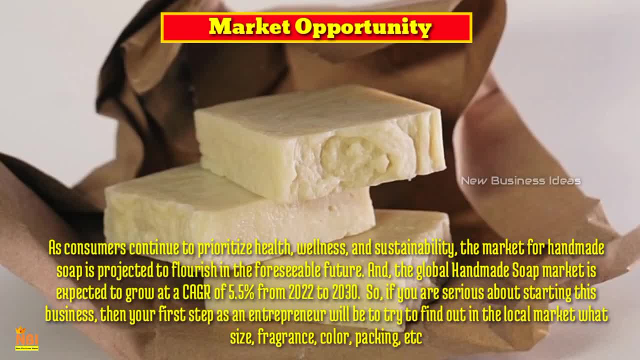 starting this business, then your first step as an entrepreneur will be to try to find out in the local market what is the best way to start this business, What are the best options available and why. In this scenario, the разбattling of the market will involve. 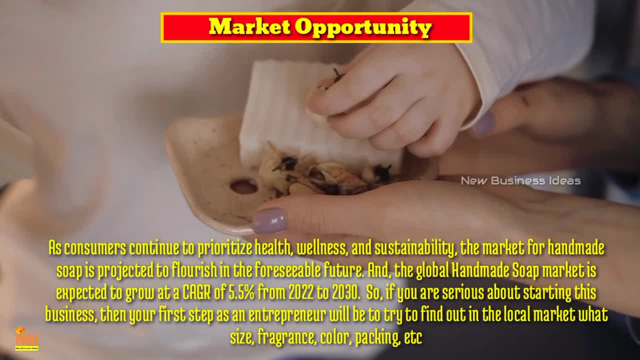 teachers, professionals and publishers. To this end, the consumer will have to identify what size, fragrance, colour, packing etc. of soap the regular users prefer. Apart from this, the entrepreneur may also need to observe the age group, income level, gender, etc. 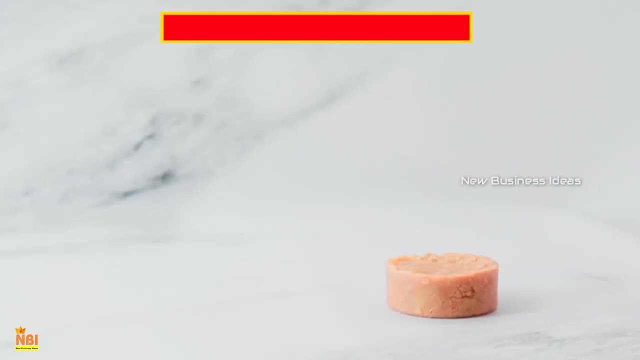 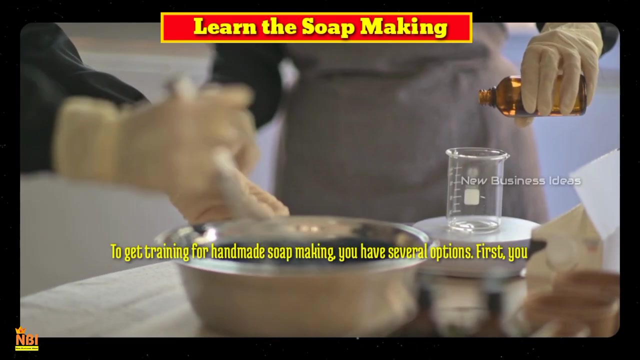 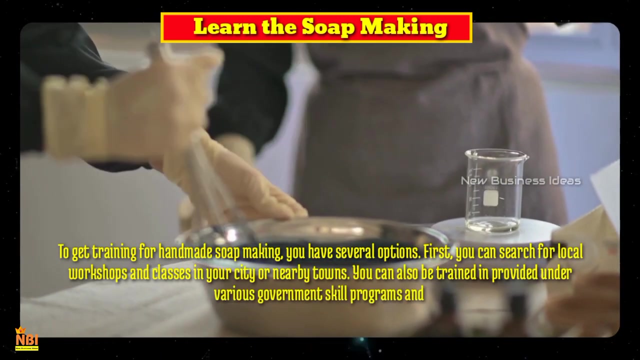 of the people living in that particular area: LEARN THE SOAP MAKING PROCESS Before any entrepreneur can sell the soap manufactured in his own manufacturing unit. if he has no knowledge of the soap making business, he will have to acquire expertise in it. To get training for handmade soap making, you have several options. 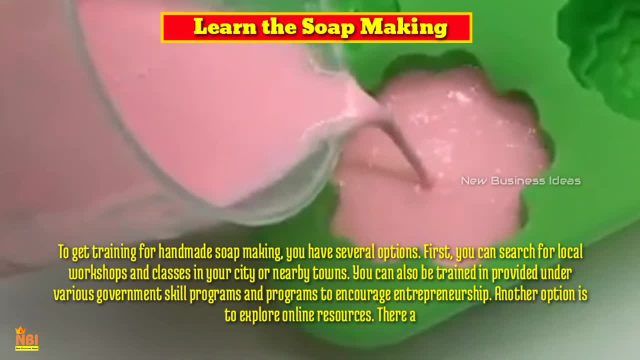 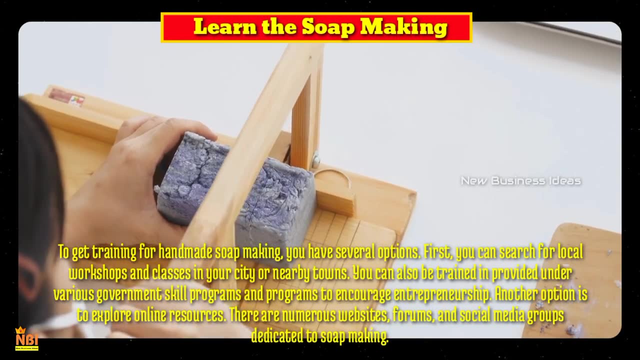 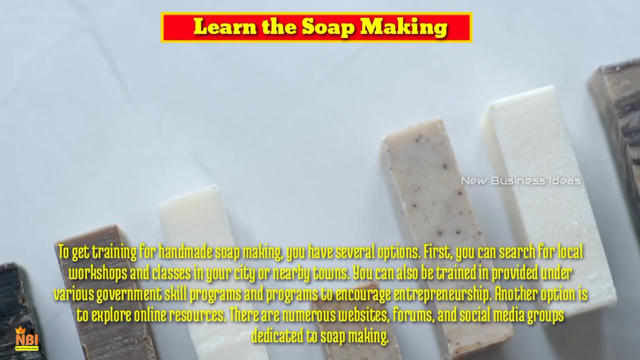 First, you can search for local workshops and classes in your city or nearby towns. You can also be trained to provide under various government-skilled programs and programs to encourage entrepreneurship. Another option is to explore online resources. There are numerous websites, forums and social media groups dedicated to soap making. 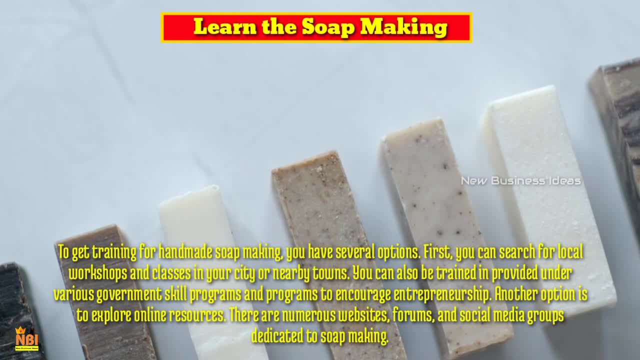 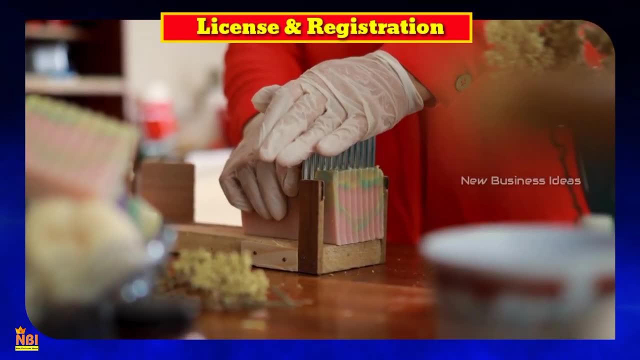 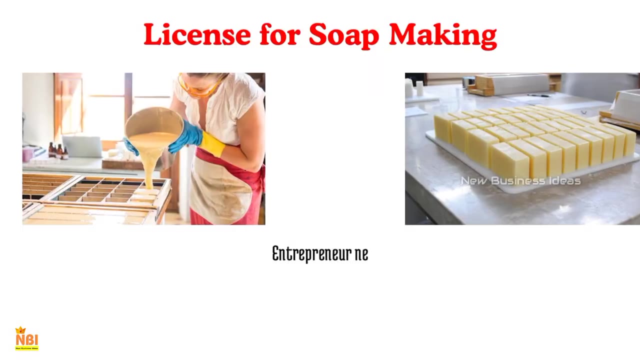 So you can learn there the basics of soap making, including choosing ingredients, the cold process and essential safety precautions, License and Registration for Handmade Soap Making. Before starting any business, it should be converted into a legal entity like a private limited company, limited liability company or partnership company. 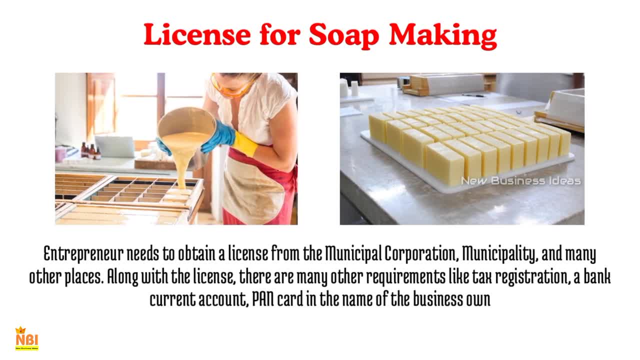 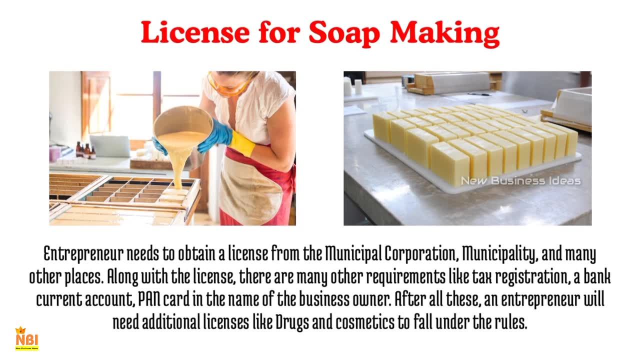 All small businesses in our country are registered and run in partnership form. Apart from this, an entrepreneur needs to obtain a license from the municipal, corporation, municipality and many other places. Along with the license, there are many other requirements like tax registration. 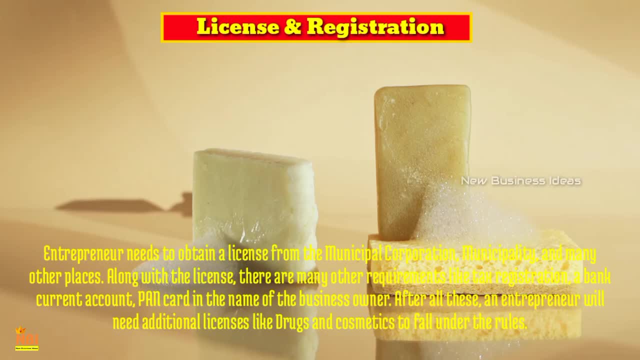 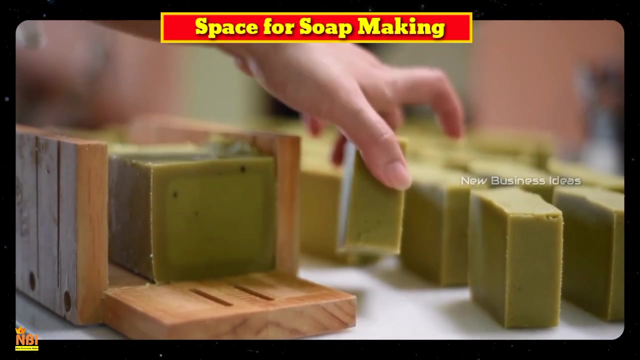 registration, a bank current account, PAN card in the name of business owner. After all these, an entrepreneur will need additional licenses, like drugs and cosmetics, to fall under the rules. Space for Soap Making: The space required for handmade soap production varies depending on the size of the operation. 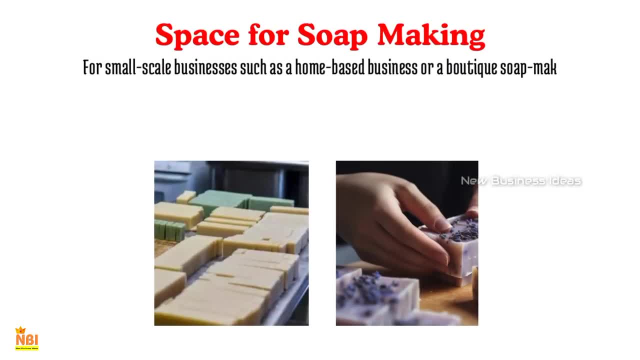 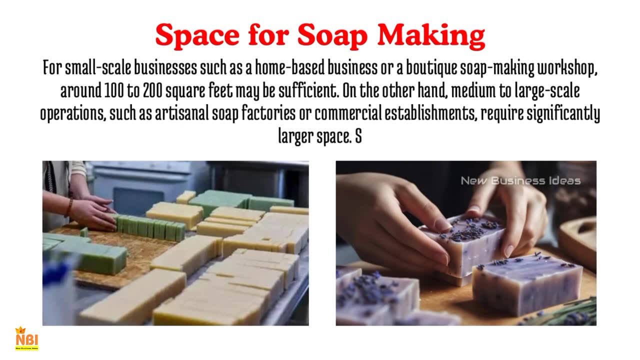 For small-scale businesses, such as home-based businesses or a boutique shop making workshop, around 100 to 200 square feet may be sufficient. On the other hand, medium to large-scale operations, such as artisanal soap factories or commercial establishments, require significantly larger space. 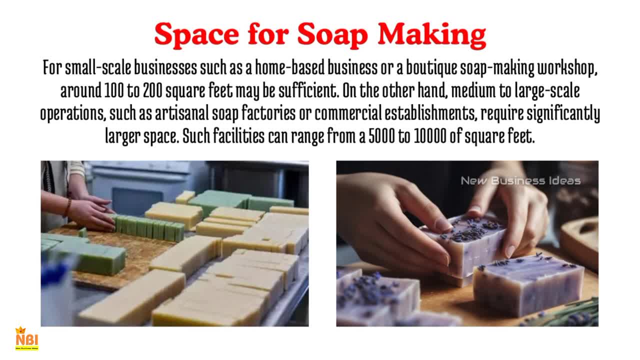 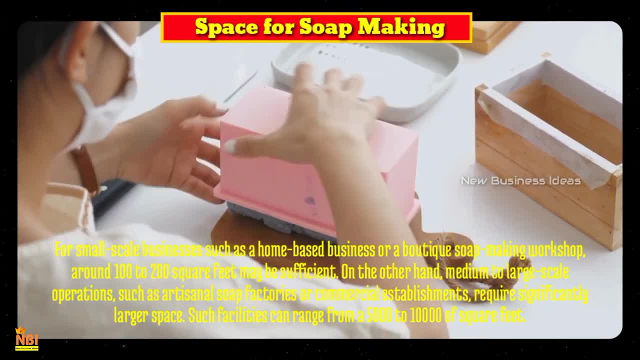 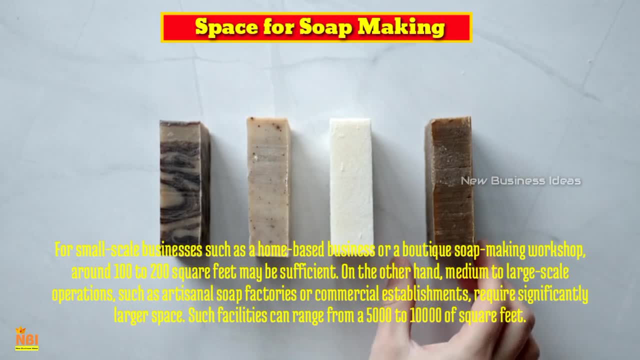 Such facilities can range from a few thousand to tens of thousands of square feet to accommodate multiple manufacturing plants, curing areas, storage facilities and administrative space. Also, adequate ventilation, water supply and compliance with local health and safety regulations are important considerations for any handmade soap manufacturing location. 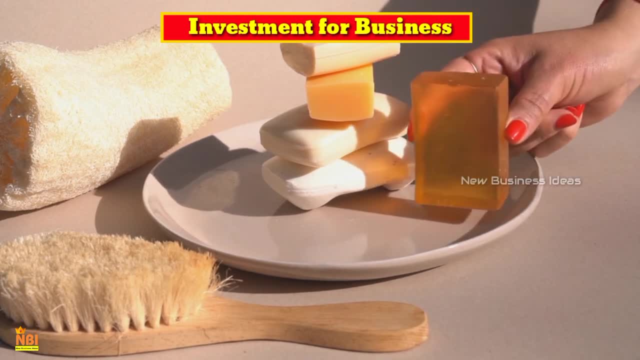 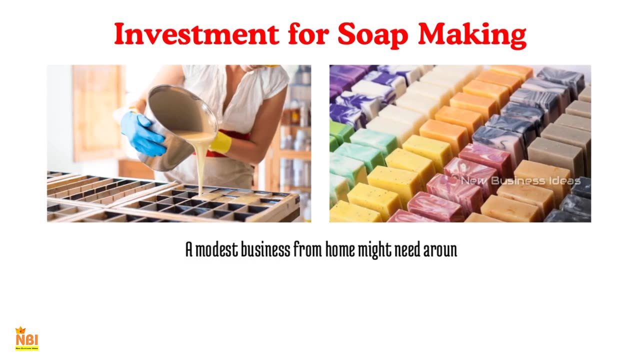 Investment for Handmade Soap Making. Now the next step is to create a home for handmade soap. The next step of the entrepreneur should be to arrange finance for his business, and the investment required for the business will depend on the size of the business and production capacity. 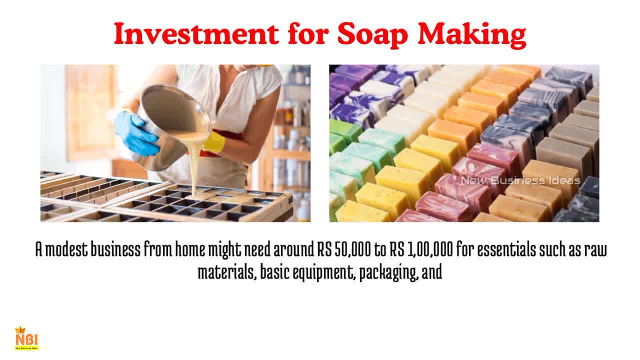 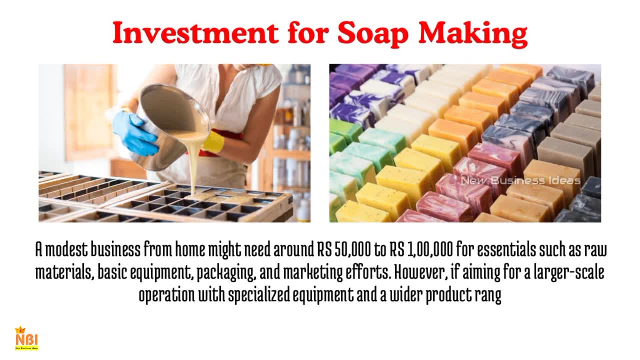 A modest business from home might need around 50,000 to 1 lakh rupees for essentials such as raw materials, basic equipment, packaging and marketing efforts. However, if aiming for a larger-scale operation with specialized equipment and a wider product range, the investment could range from 2 lakh to 5 lakh or more. 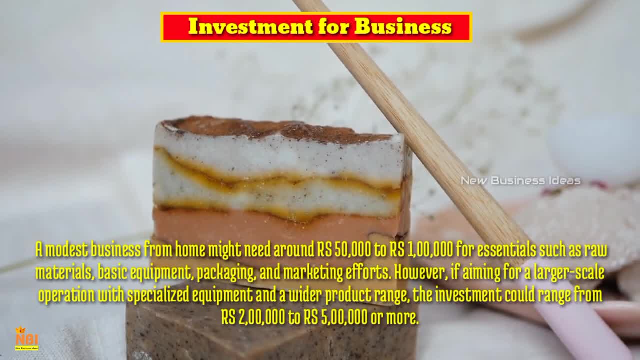 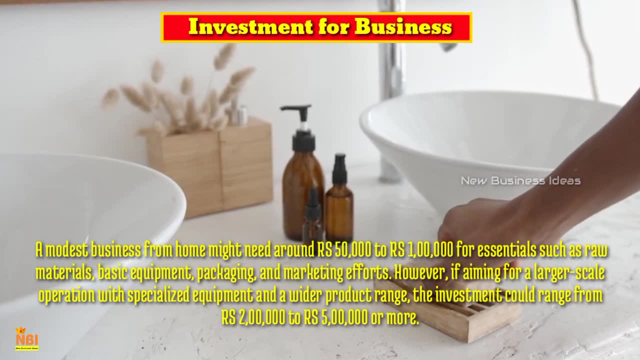 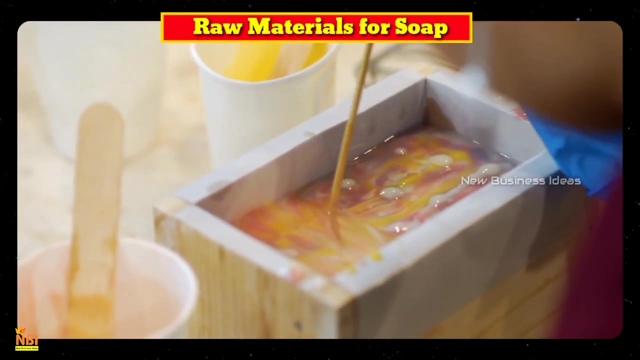 Additionally, marketing and distribution costs should be factored in to ensure a successful launch and sustainable growth in the competitive hand-made soap market. So it's crucial to allocate funds for quality ingredients and compliance with safety and hygiene standards. Raw Materials for Handmade Soap Making. 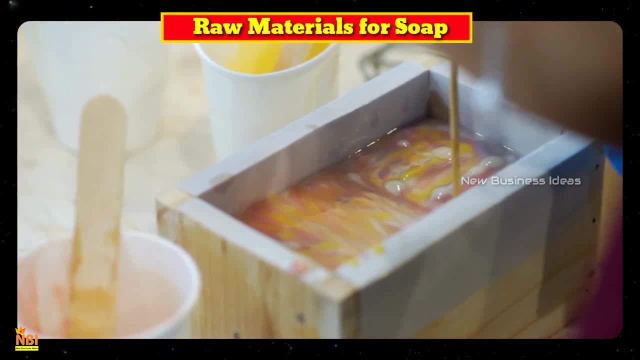 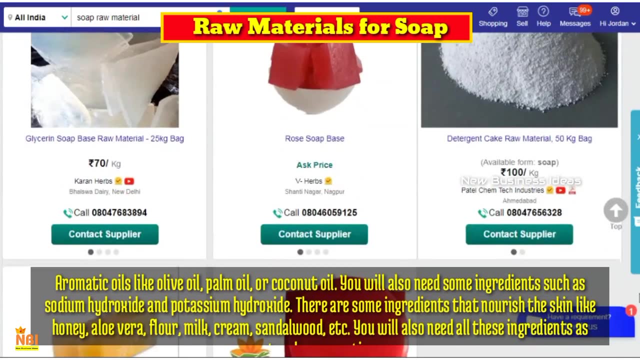 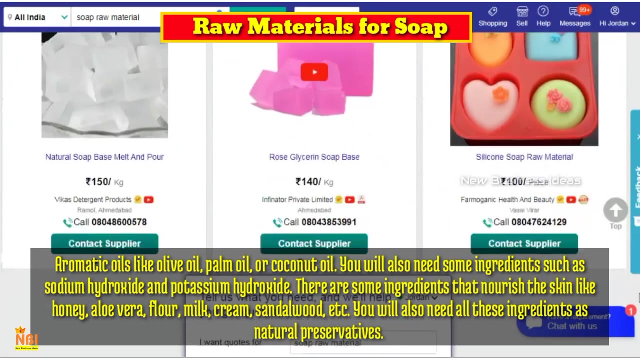 The following list of the raw materials required to make soap: Aromatic oils like olive oil, palm oil or coconut oil. You will also need some ingredients such as sodium hydroxide and potassium hydroxide. There are some ingredients that nourish the skin, like honey, aloe vera, flour, milk, cream, sandalwood, etc. 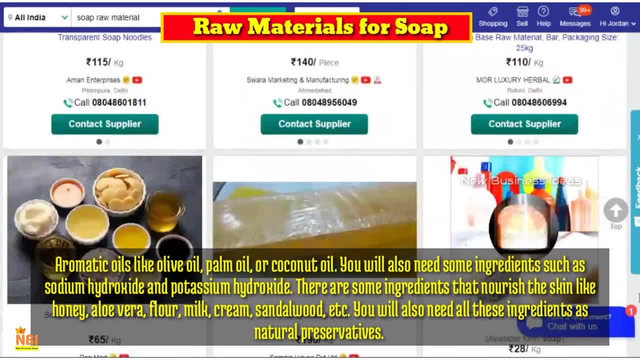 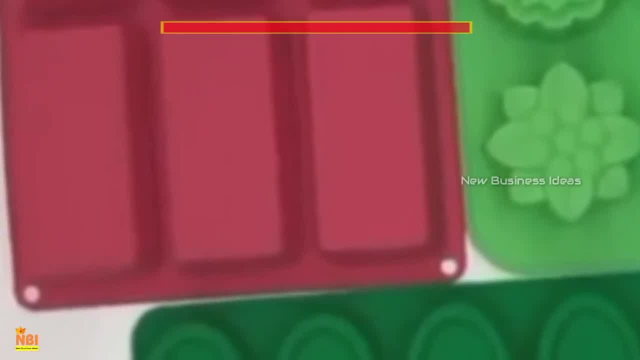 You will also need all these ingredients as natural preservatives Also need some artificial fragrances and artificial colours. moulds, containers and packaging materials. Tools and Equipment for Handmade Soap Making. Following are the tools and equipment you will require to begin working at home. 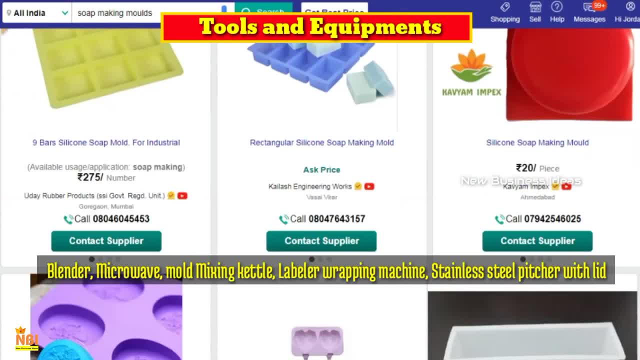 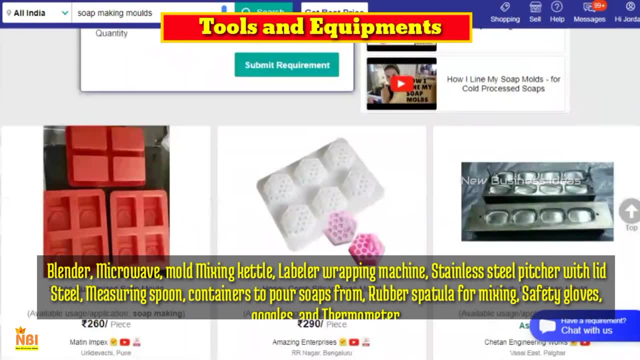 Blender, Microwave Mould, Mixing Kettle, Labeler, Wrapping Machine, Stainless Steel Pipe. A Pitcher with Lid, Steel Measuring Spoon, Containers to Pour Soap from Rubber Spatula for Mixing. Safety Gloves, Goggles and Thermometer. 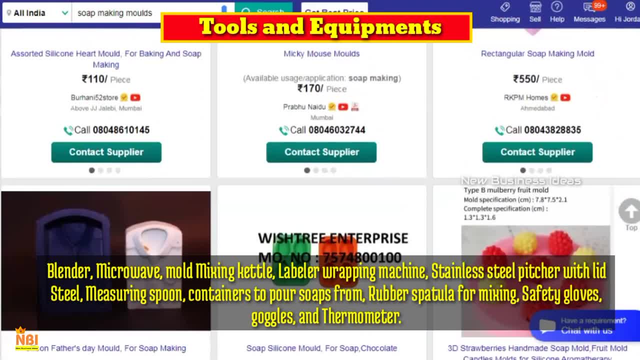 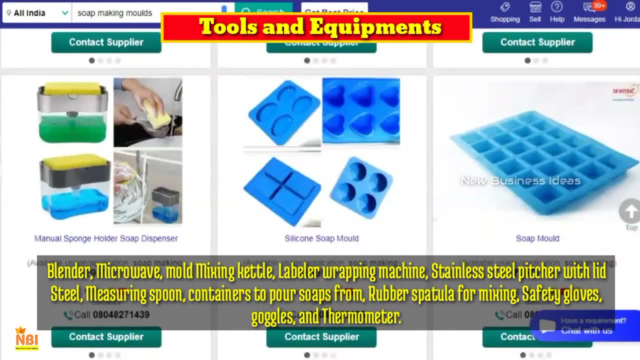 You can buy it from your local wholesale market, Or if you want to get all of them at home, then you will find many types of machines at different prices on India Mart and Alibaba websites. You will also get the contact number of the dealers of the machine. 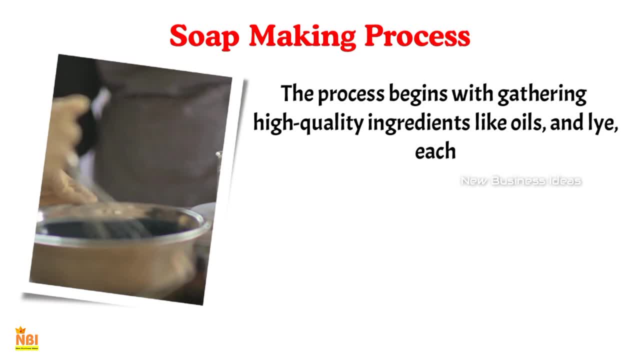 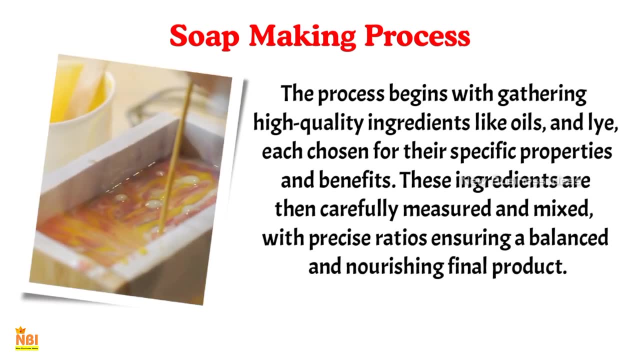 Handmade Soap Making Process. Creating handmade soap is a meticulous craft that combines science and artistry. The process begins with gathering high-quality ingredients like oils and lime, each chosen for their specific properties and benefits. These ingredients are then carefully measured and mixed with precise ratios, ensuring a balanced and nourishing final product. 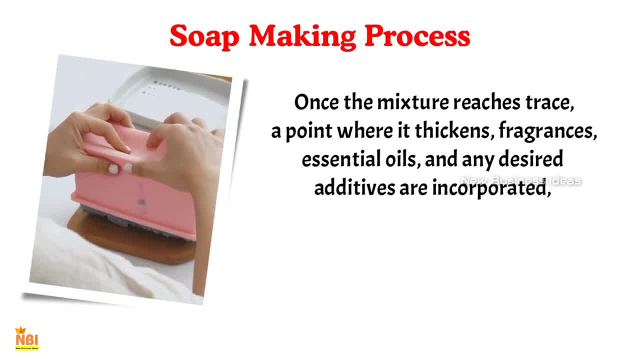 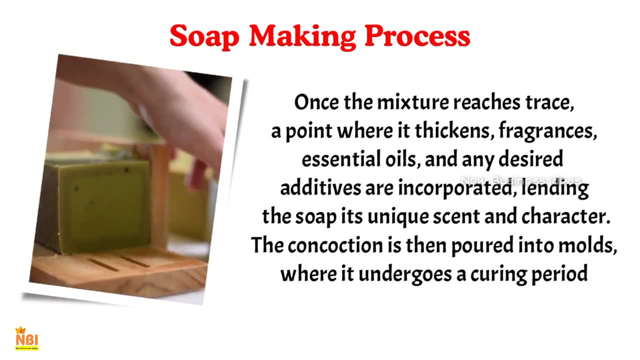 Once the mixture reaches traces, a point where it thickens, fragrances, essential oils and any other required additives are incorporated, lending the soap its unique scent and character. The concoction is then poured on the surface of the soap for it to absorb the oil and the soap. 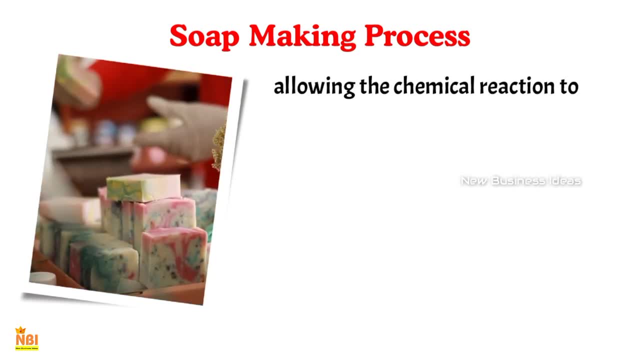 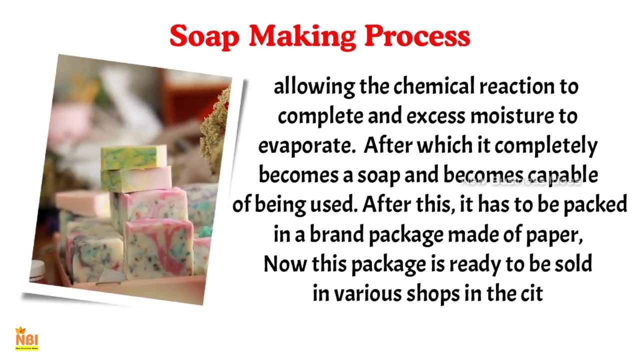 into molds, where it undergoes a curing period allowing the chemical reaction to complete and excess moisture to evaporate, after which it completely becomes a soap and becomes capable of being used. after this, it has to be packed in a brand package made of paper. now this package is: 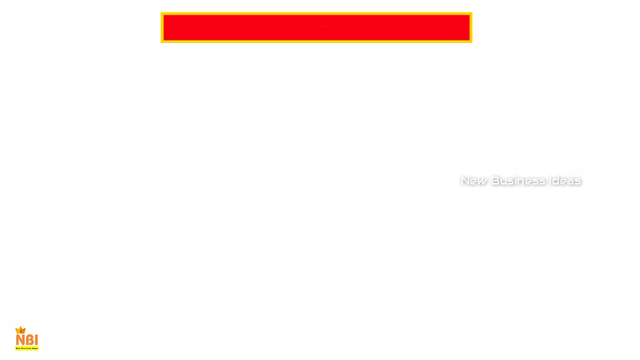 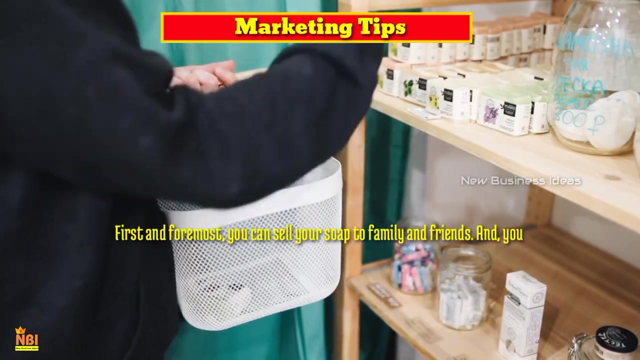 ready to be sold in various shops in the city. marketing for handmade soap. in today's time, if any product has to be sold, then marketing that product is very important. first and foremost, you can sell your soap to family and friends and you can also promote by visiting hotels, spas, resorts. 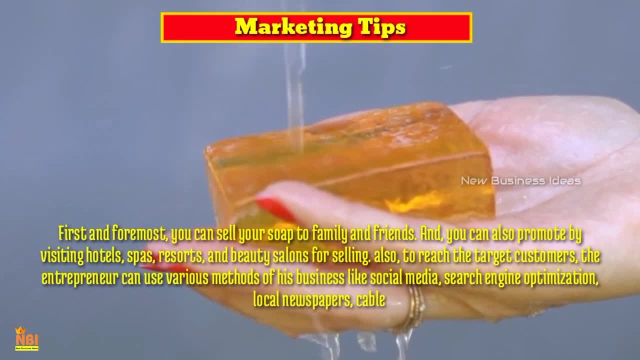 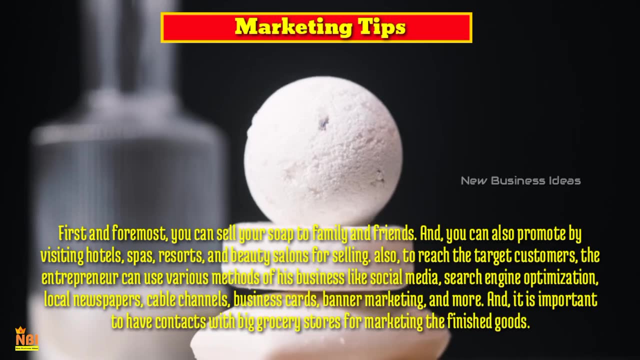 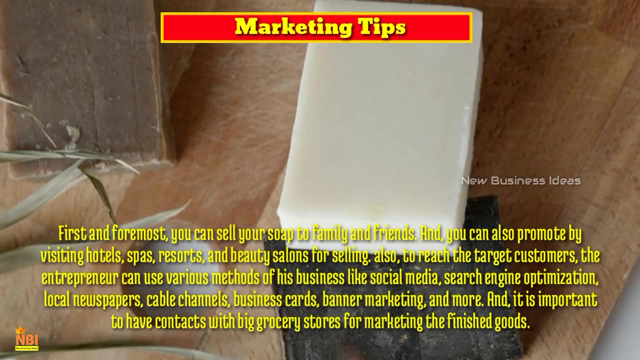 and beauty salons for selling. also, to reach the target customers, the entrepreneur can use various methods of his business, like social media, search engine optimization, local newspapers, cable channels, business cards, banner marketing and more. and it is important to have contacts with big grocery stores for marketing the finished goods, because it is from here that small shopkeepers 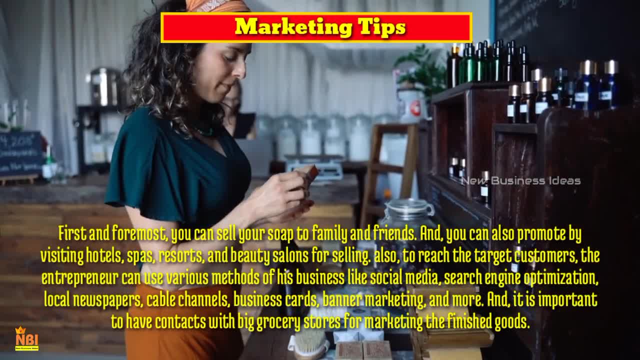 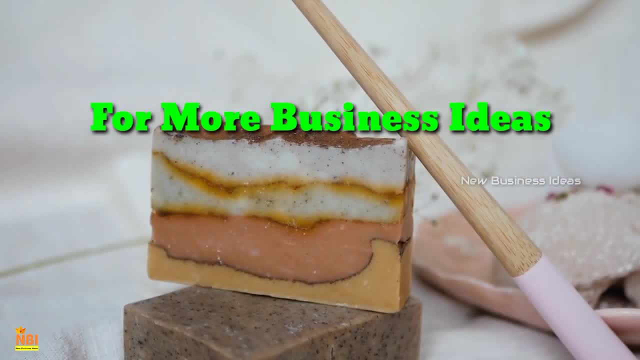 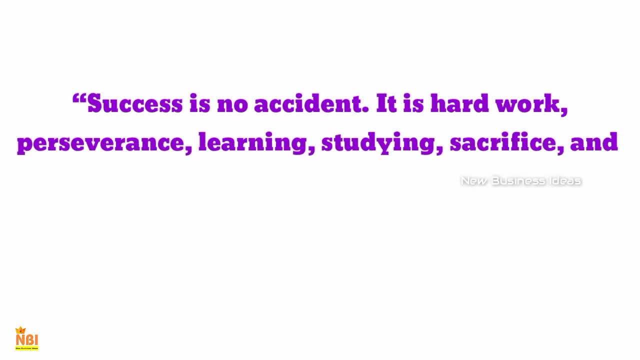 buy and sell soap, so attractive packages and limited period offers can help in capturing the market. if you want to know more information about this business, please check our website and the link in the video description. we hope in this video it helped you to initiate your own business. if you like the video, please give it a like and comment. 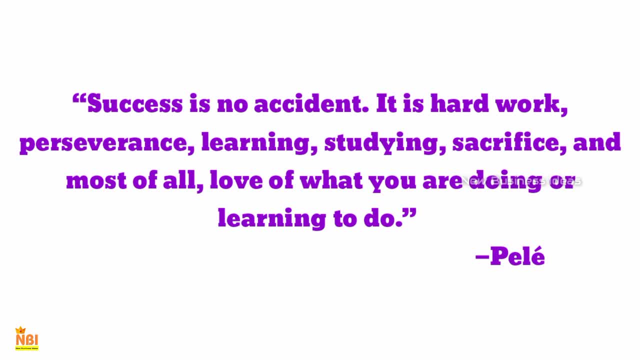 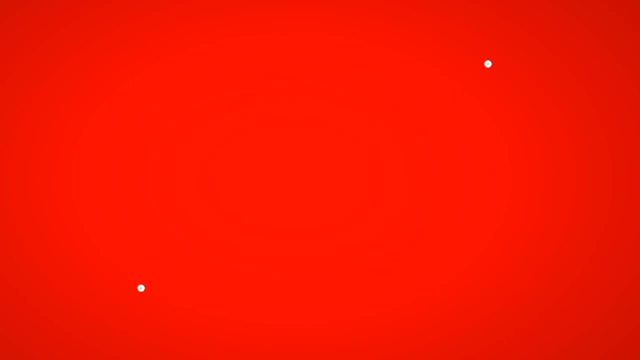 thank you for watching friends for more business ideas. subscribe to new business ideas. so you.